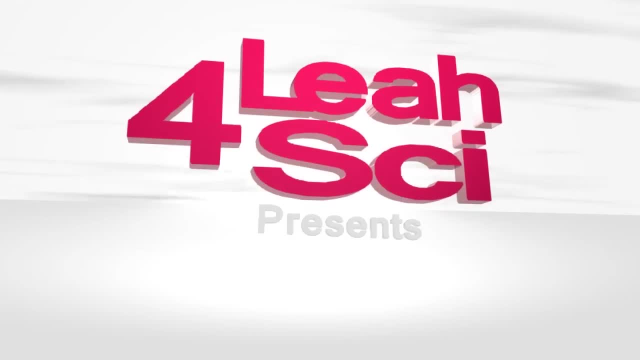 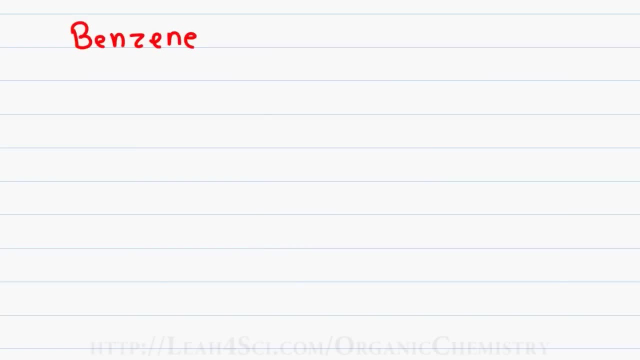 Leah here from leah4scicom, and in this video I will show you how to name aromatic compounds. Benzene is the most common aromatic compound that you will see in organic chemistry and can be represented as six carbons in a ring with alternating double bonds and a single. 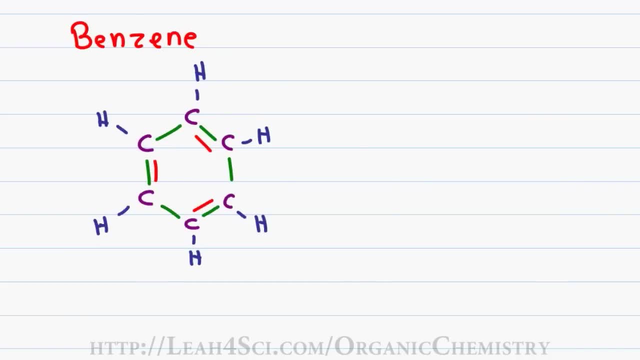 hydrogen on each carbon. This structure can be simplified by drawing a hexagon with three pi bonds, recognizing that the pi bonds can resonate in the molecule. This can be further simplified by drawing a circle in the center of your hexagon to show the resonating pi electrons. 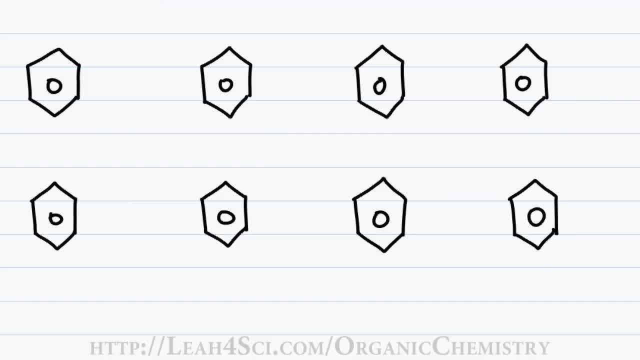 Aromatic compounds were studied long before their names were formalized, and so the IUPAC name reflect their common names. Your professor will likely have you memorize a very long list. I will show you some here, but you can download a more detailed list. 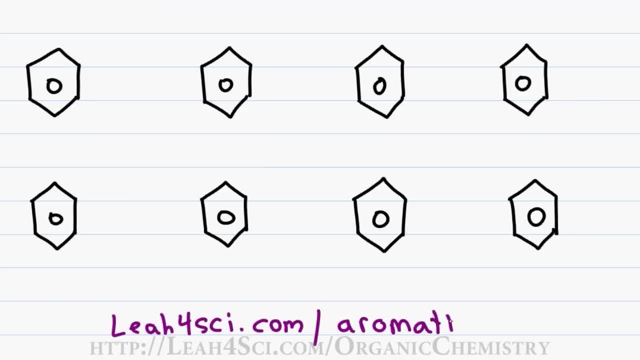 on my website at leah4scicom: slash aromatics. When you have an OH coming off your benzene ring, you can recognize this as an alcohol. that would be named benzinol but is commonly called phenol. When you have a CH3 or methyl group coming off your benzene ring, 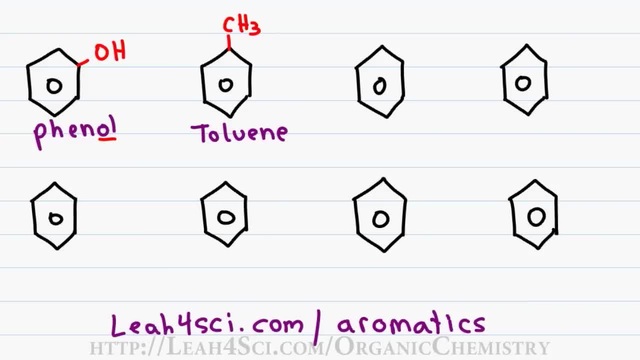 this methylbenzene is actually called toluene. When you have an NH2 on your ring, this is benzinamine, commonly called aniline. An OCH3 or methoxy substituent off your benzene ring would be methoxybenzene, but is called anisole, A carboxylic acid off your benzene ring will. 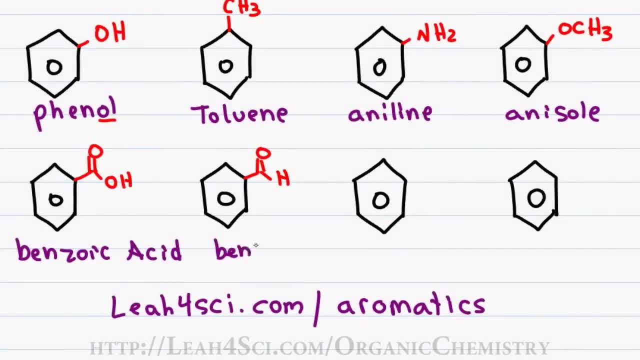 be benzoic acid and an aldehyde will give you benzaldehyde. When you have a vinyl group, which is two carbons double bound to each other, coming off your benzene ring, this would be called vinyl benzene, but has the name styrene, And we'll finish off with an. 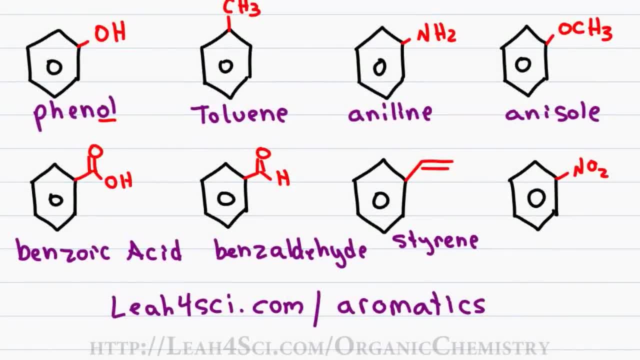 interesting example: When you have NO2 off your ring, this is called nitrobenzene, and what's interesting about this is, even though NO2 has no charge, when you draw it out you have a nitrogen coming off the ring, double bound to one oxygen and single bound to a second- The single bound oxygen. 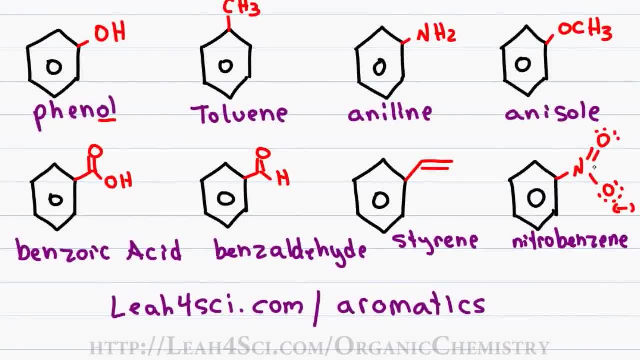 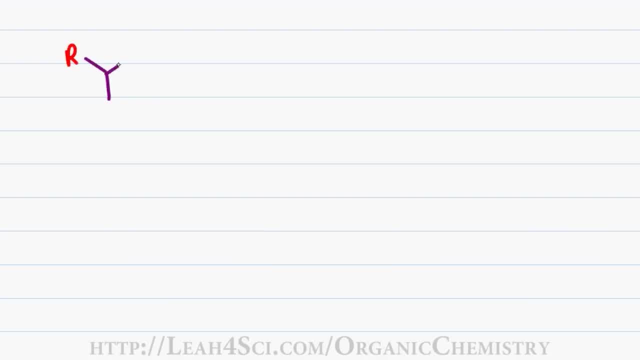 alone pairs with a formal charge of negative one, and your nitrogen has a formal charge of positive one, which plays a major role in EAS reactions. When you have benzene as a substituent off a larger molecule, this is a phenyl group. Students often confuse the phenyl group with a benzyl group. 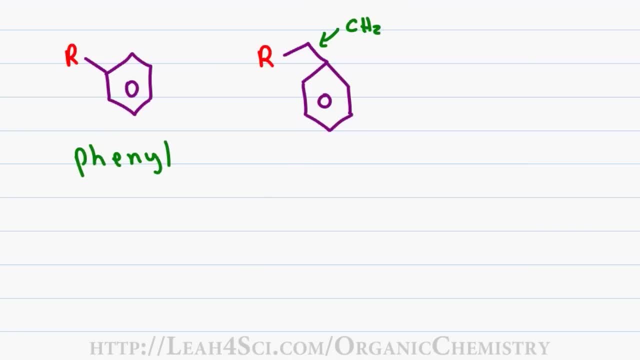 which actually has a CH2 coming off your parent chain, and then the benzene ring. Phenol is another molecule often confused by name. however, phenol is an alcohol and phenyl is your benzene substituent. Because the benzene ring is slightly complicated to draw, you may often see the substituents. 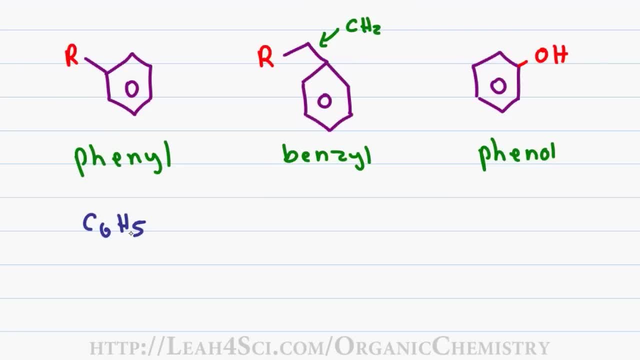 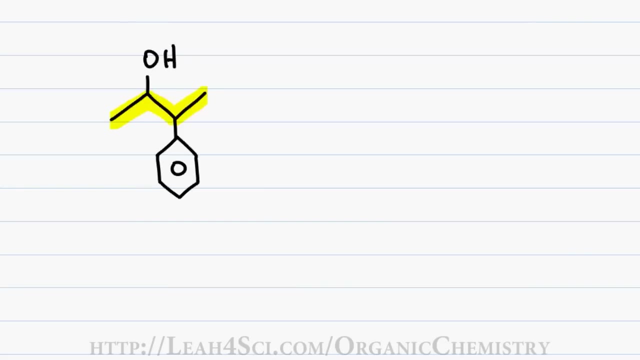 simply listed as C6H5 for phenol, which is simply a benzene group, or C7H7 for benzol, which is a toluene group. We'll use this molecule for our first example. We have a parent chain that has a total of four carbons which we can name from. 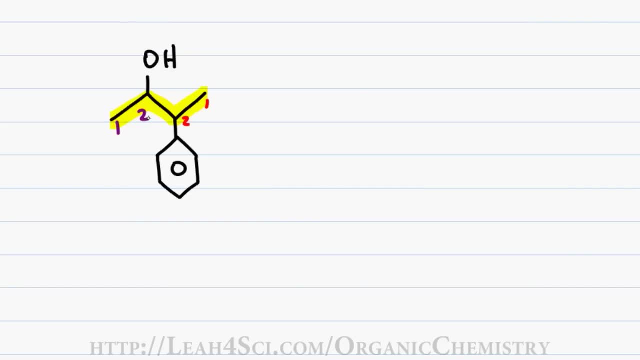 the right giving benzene a number two, or named from the left giving the alcohol number two. Since there is a presence of NO2 in thecrossing hiccup, jadi, we are hoping that NO2 will stay there. A family strand to this gasoline is Tollazoint and zero dalgona. Some people may beável que este es un необходимо de era. 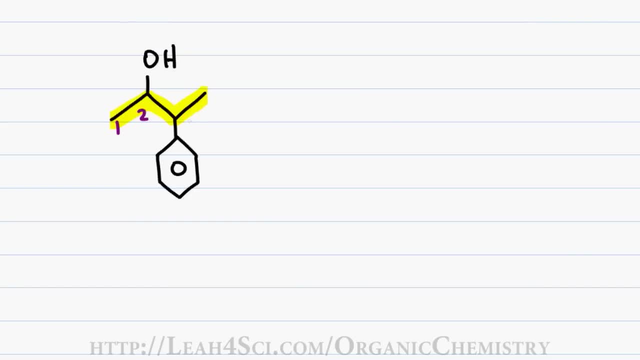 Since OH has a higher priority than the phenyl group, we have to number from the left and get a total of 4 carbons. for a first name of bute, Only single bonds in the parent chain gives me a last name of ane and an OH functional. 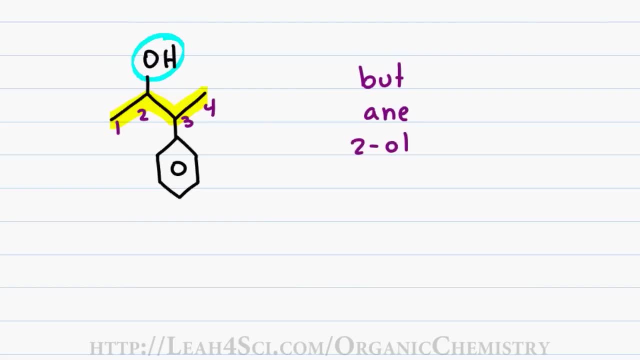 group on carbon 2 gives me the suffix 2-ol And, last but not least, having a benzene ring coming off. carbon 3 gives me the substituent 3-phenyl. I pull the 2 from ol in front of the parent name, allowing me to drop the e and ane for. 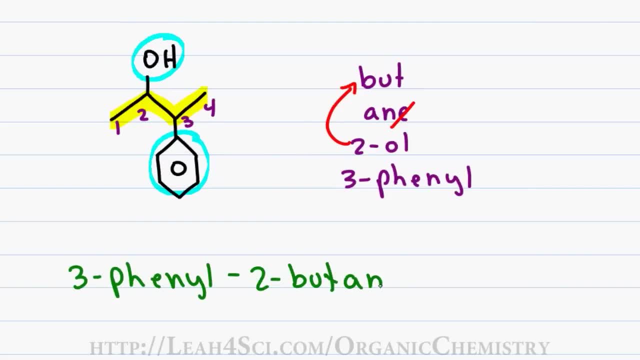 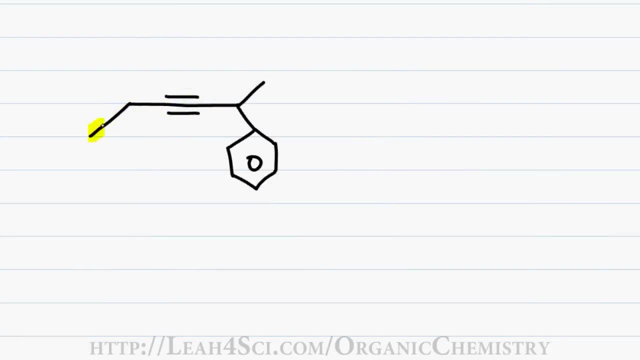 a final name of 3-phenyl-2-butanol. In this example, we have both a triple bond and a benzene ring on my parent chain. Again, I start by identifying and highlighting the parent chain and then number it from the direction that gives me the total lowest set of numbers. 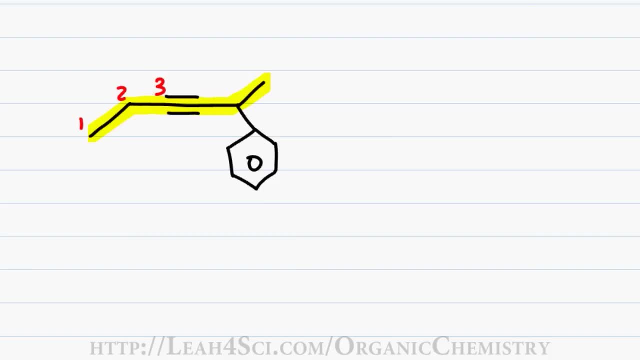 If I number from the left, I hit the triple bond on number 3.. If I number from the right, I hit benzene on number 2. And so I number from the right for a total of 6 carbons and a first name of it. 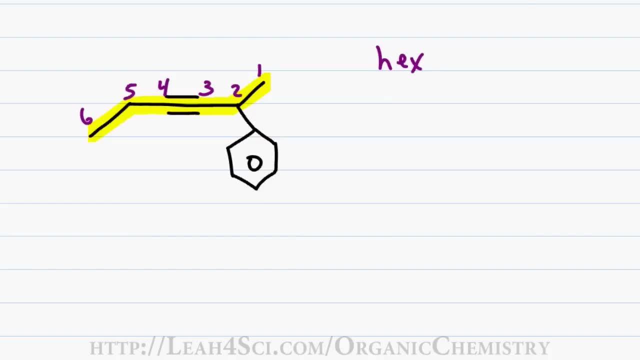 A triple bond on the parent chain on carbon 3 gives me the last name of 3-yne and a benzene substituent off carbon 2 gives me the prefix 2-phenyl. I can pull the number 3 in front of hex for a final name of 2-phenyl-3-hex-yne. 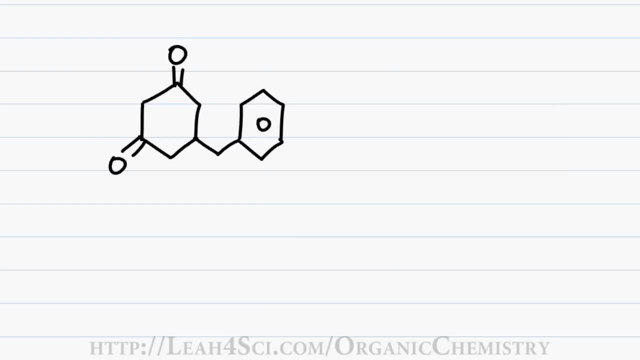 Don't let the complexity of this example fool you. We simply have a parent chain with multiple functional groups and substituents, and so we'll apply the puzzle pieces slowly to make sure we get it right. Don't let the complexity of this example fool you. 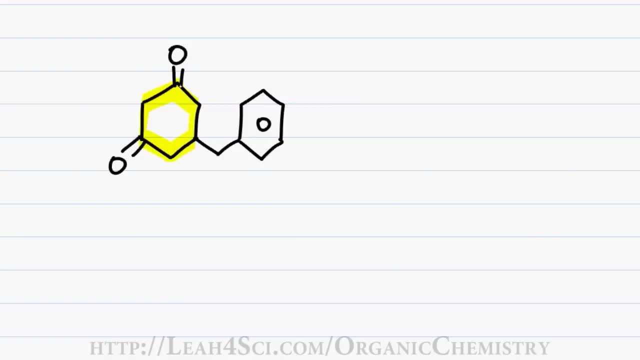 We simply have a parent chain with multiple functional groups and substituents, and so we'll apply the puzzle pieces slowly to make sure we get it right. Don't let the complexity of this example fool you. We simply have a parent chain with multiple functional groups and substituents, and so we'll 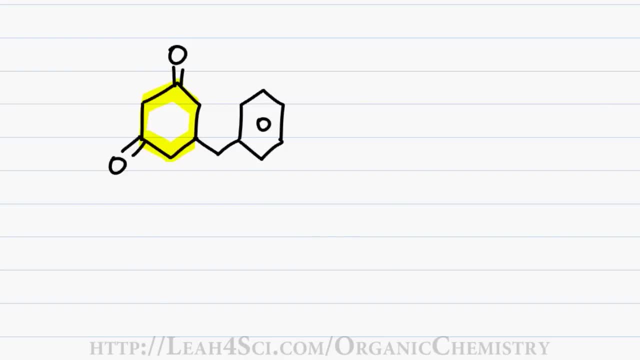 apply the puzzle pieces slowly to make sure we get it right. The parent chain will be the cyclohex-yne and since the ketone is highest priority, we have to ensure that the ketones get the two lowest numbers. I can start from one ketone, work my way to the second, giving them the numbers 1 and 3. 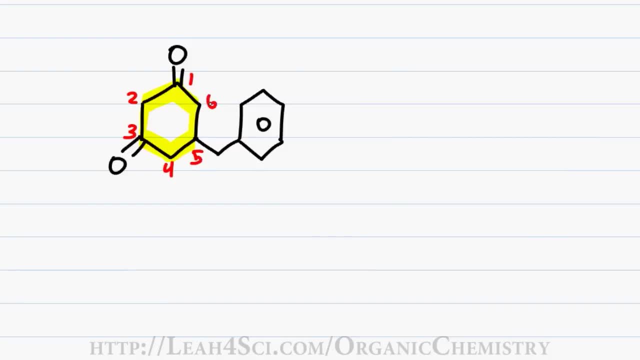 and continue in that direction, for a total of 6 carbons in my parent chain and a first name of hex. Since the 6 carbons occur in a ring, I have the prefix cyclo and only single bonds in the ring gives me a last name of yne. 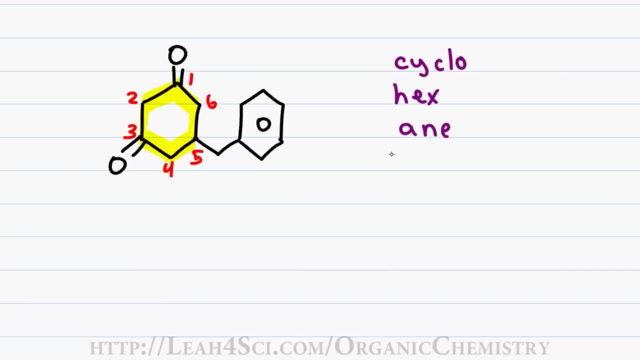 Having two ketone functional groups on the molecule gives me the suffix 1,3-dione, where 1 and 3 tell me where each one occurs and di tells me that I have two, While the substituent is a benzene ring. this is not a phenyl group, because I also have 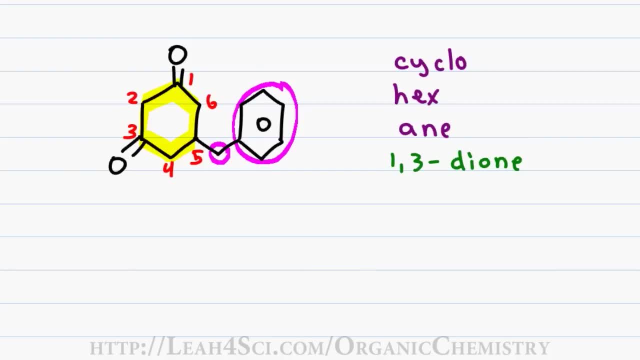 the CH2 connected to it as one larger substituent. This gives me the prefix of 5-benzyl rather than 5-phenyl. I pull the numbers 1 and 3 in front of the word cyclo for a final name of 5-benzyl: 1-phenylyl. 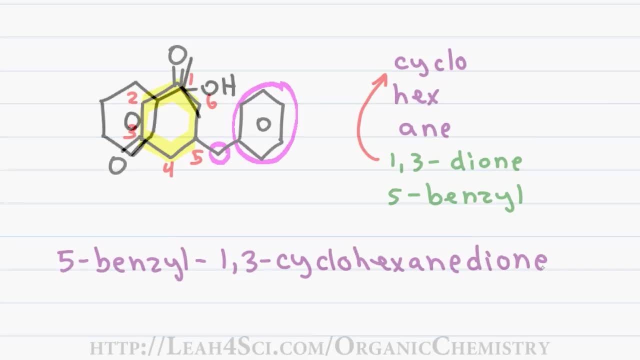 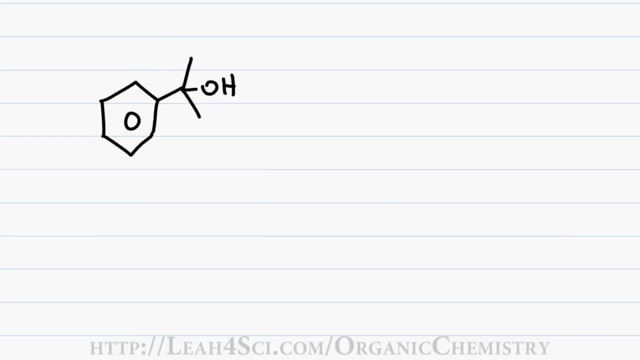 1,3-cyclohexane-dione. This example was shown to me by a confused student who wasn't sure how to find the parent chain. While it looks tricky, simply identify the central carbon atom and see if you can find the longest carbon chain. 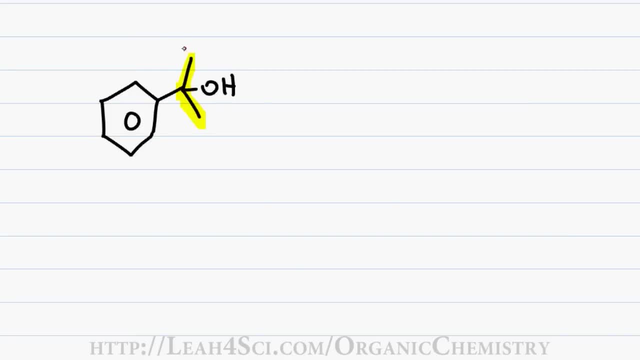 In this case we have a symmetrical molecule with a total of 3 carbons for a first name of prop. Only single bonds on the carbon gives me a last name of ane, and an OH functional group on carbon 2 gives me the suffix 2-phenylyl. 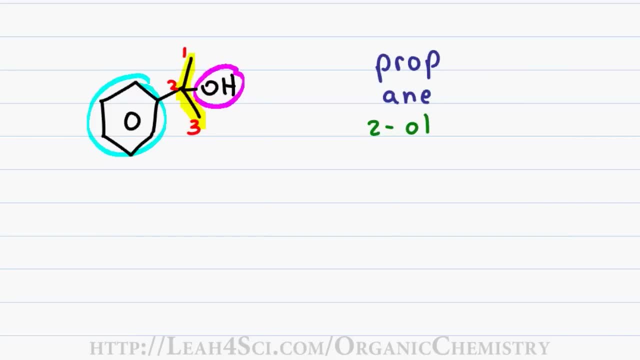 Having the benzene substituent on carbon 2 gives me the prefix 2-phenyl. I pull the 2 in front of the word prop, drop the e in ane and get a final name of 2-phenyl-2-propanol. 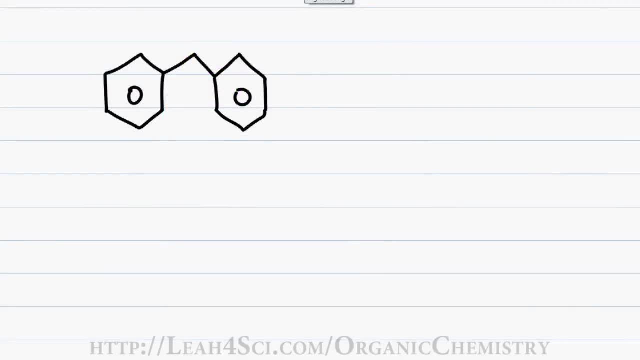 We'll end part 1 with an interesting example. At first glance, this looks like a complicated molecule. however, if you look closer, you'll notice that your parent chain has one single carbon. This one carbon gives me a first name of 2-phenylyl-2-propanol.